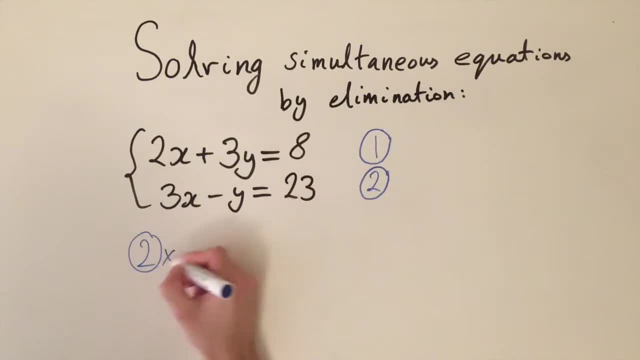 take the second equation and we're going to multiply it by 3. so this is just to keep track of what we're doing. so we're taking the second equation, multiply both sides by 3. we're gonna get: 3 times 3x is 9x, 3 times minus y is minus 3y and 3. 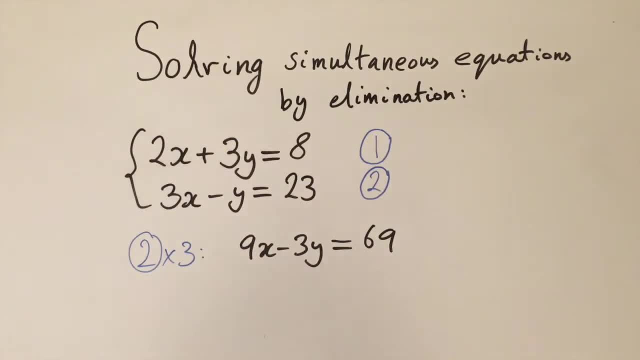 times 23 is 69, and I'm going to label this equation number 3, and I'm going to label this equation number 3 and I'm going to label this equation number 3.. This equation has identical solutions to equation 2.. We've just multiplied both sides. 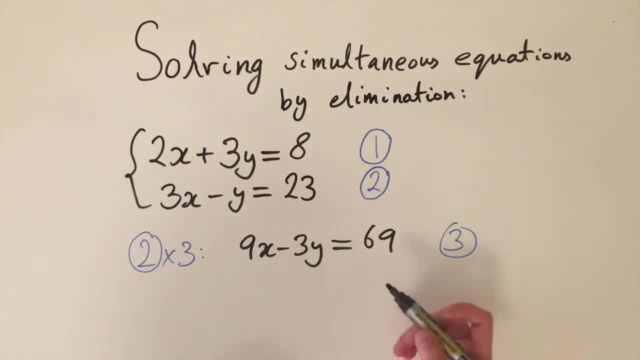 by the same number. so we're not changing anything about the equation. And now you can see that in equation 3 and in equation 2, we have two terms involving 3y. So now what we're going to do is we're going to add equation 1 and equation 3, and then the 3y terms are: 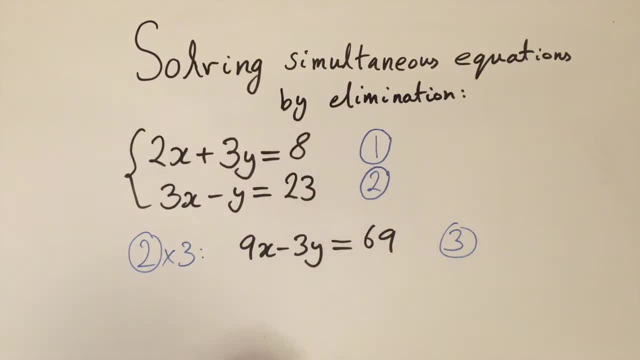 going to cancel out, So I'll just write this over here: We're going to add equation 1 and equation 3.. So we have to add the left-hand sides together and the right-hand sides together. So if we add 2x plus 3y, this is from equation 1, and we're going to add 9x minus 3y And then 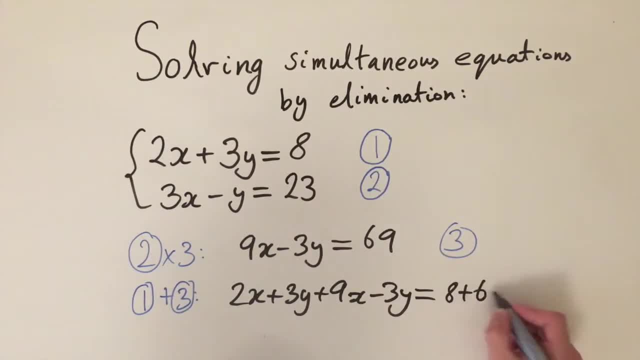 on the right-hand side. we're going to add 8 and 69 together, And this simplifies as 77.. Okay, so now the 3y's are going to cancel out, And we've just got an equation involving x's, So let's collect. 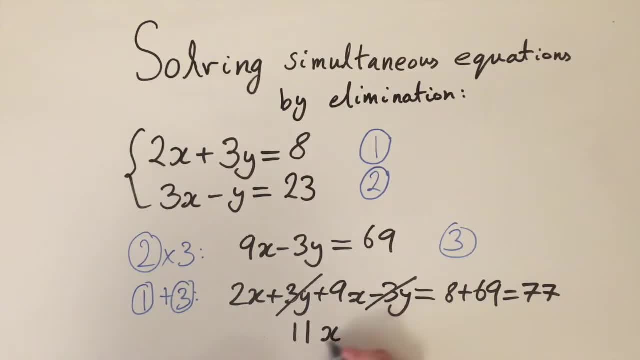 the terms: We have 11x on the left-hand side and we have 77 on the right-hand side. And now this is just going to solve by dividing both sides by 11. We're just going to get: x is equal to 7.. So this is half of the solution. 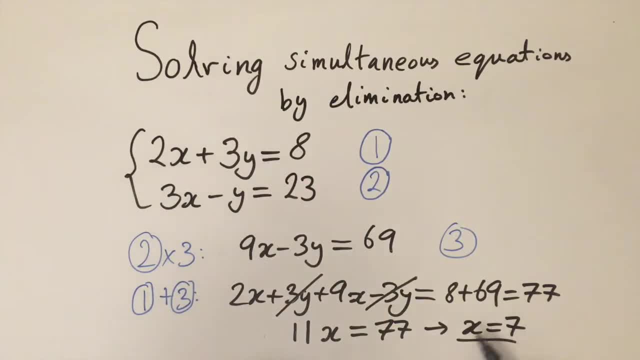 Now we also want to know what value of y that corresponds to this value of x also solves both equations. So what we're going to do is substitute this value of x into either one of these equations. It doesn't matter which one. We're going to go for the second one, because there's only 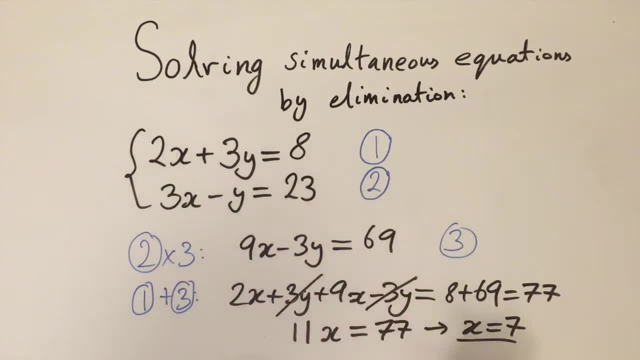 one coefficient of y, And that's going to make it a bit simpler. So let's go up here And we're going to substitute x is equal to 7 into the second equation. So I'm just going to write substitute into substitute in 2, just to keep track of what we're doing. And 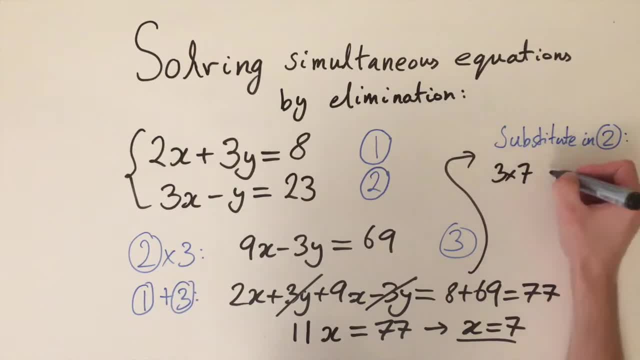 we're going to get 3 times x. x is 7, then minus y- That's what we're trying to find out- And this equals 23.. So if we just solve this, we're going to rearrange for y. Let's add y onto the right-hand side. 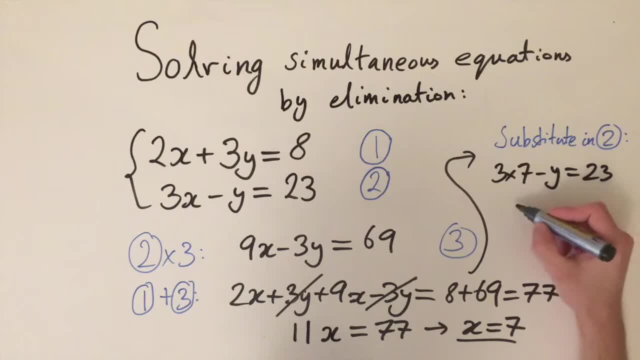 and subtract by 23.. So 3 times 7,, which is 21.. Subtract by 23 on both sides and add y onto the right-hand side, And then 21 minus 23,. that's just minus 2.. So we get that y. 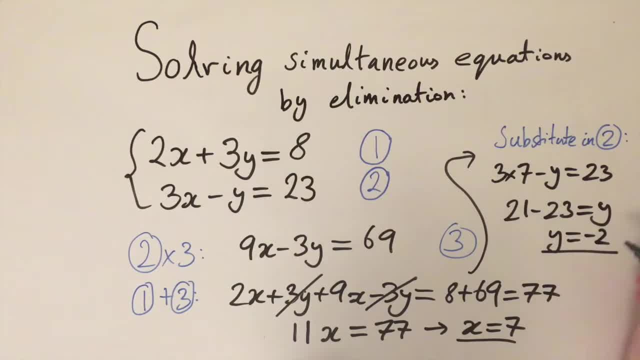 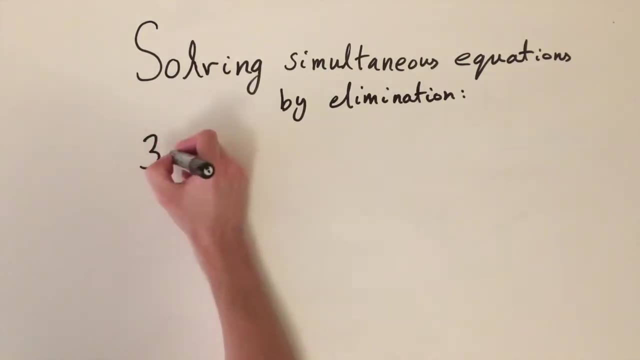 is equal to minus 2.. And this is the second half Half of the solution. So together, x equals 7 and y equals minus 2.. This forms the solution of this pair of simultaneous equations. OK, let's look at a second example. We're going to do: 3x plus 8y is equal to 33.. And 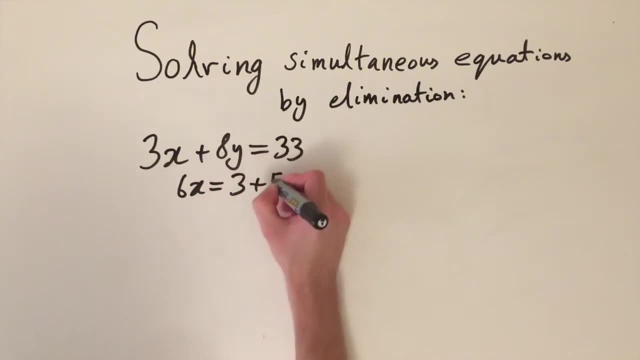 6x is equal to 3 plus 5y. So this is the second equation is now rearranged in a slightly different form. It doesn't actually matter, We're going to use the same technique. So firstly, I'm just going to label the first. 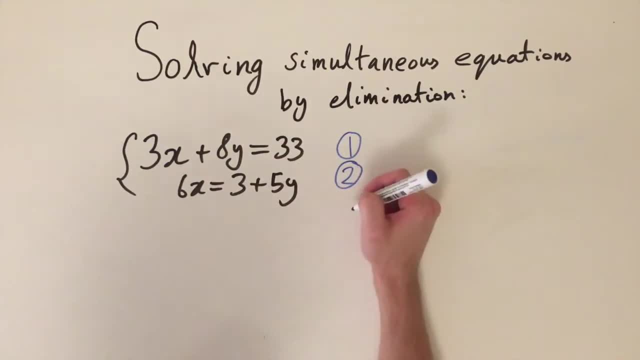 equation as equation 1 and the second equation as equation 2.. So, just as before, we want to multiply one of these equations by a number, so that the same term of one variable appears in both equations. So we could eliminate x or we could eliminate y, But we see here that 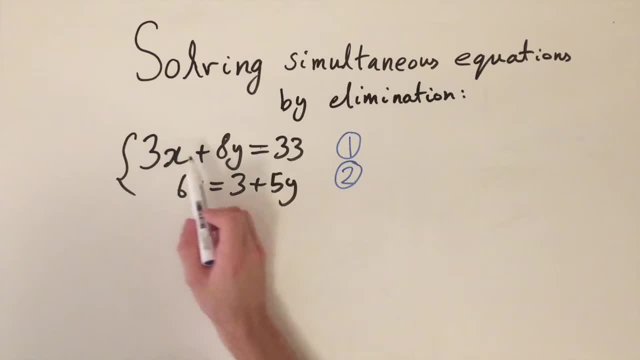 if we multiply the first equation by 2, then we're going to get 6x in both of these equations. So I'm just going to write down 2 times the first equation. And now, if we multiply 2 by the first equation on both sides, we're going to get 2 times. 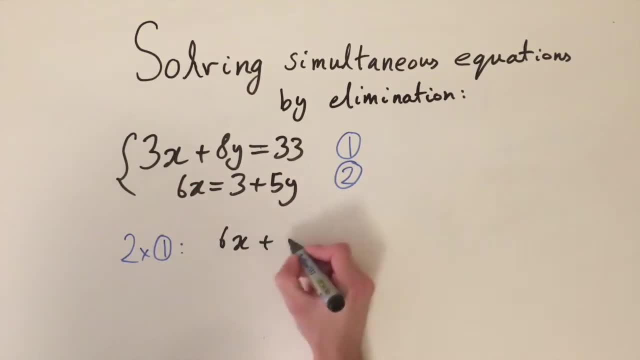 3x, which is 6x, 2 times 8y, which is 16y, and 2 times 33.. So this equals 66. And let's label this as equation 3.. So, just as I said before, this equation is identical to the first equation. So we're. 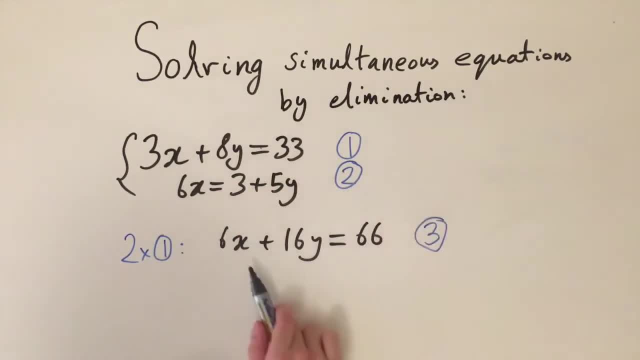 now just considering equation 2 and equation 3.. And we see that both of these equations are identical. So if we were to subtract one from the other, this term would just cancel out. So that's what we're going to do. So it doesn't matter what order we do this in. Let's do equation 2 minus equation 3.. 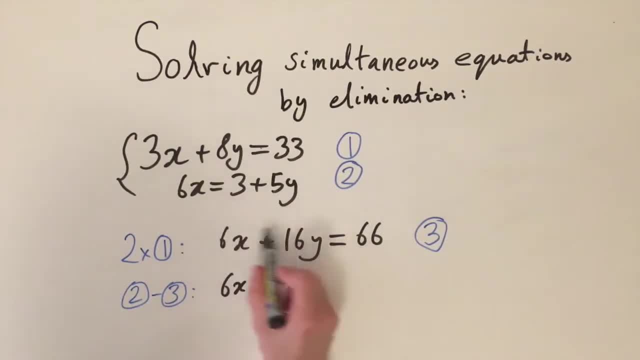 And then we get 6x on the left-hand side minus the left-hand side of equation 3.. 6x plus 16y. And then on the right-hand side we have 3 plus 5y from equation 2. And then 66. And 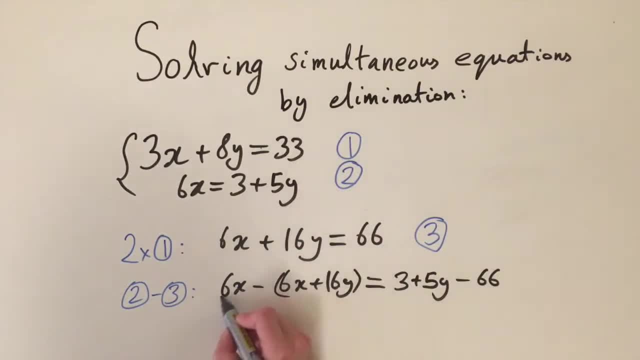 from equation 3.. So now the 6x's cancel out. You can see this, And we've just got an equation involving y which we can solve. So let's distribute the negative sign We have minus 16y is equal. 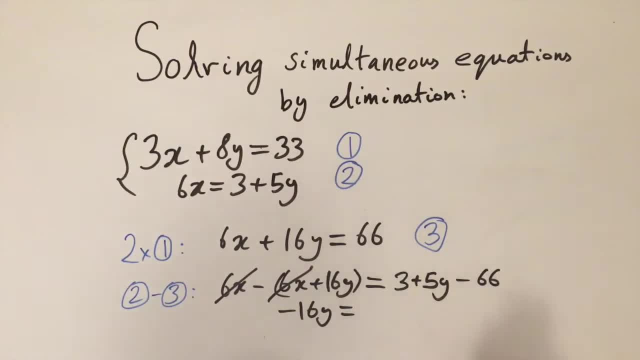 to well, 3 minus 66. That's just minus 63. So we have 5y minus 63. And now let's rearrange to find y on its own. So let's add 16y onto that side and add 63 onto this side, So we 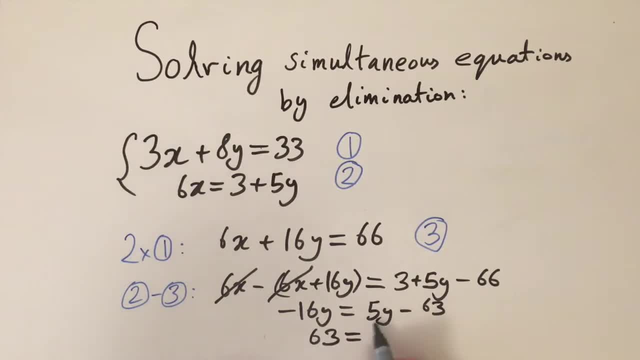 have 66.. 63 is equal to 16y plus 5y, That's 21y 16 plus 5.. And then all we have to do is divide by 21.. And 63 is 3 times 21.. So we get y is equal to 3 as our solution. Well, half the. 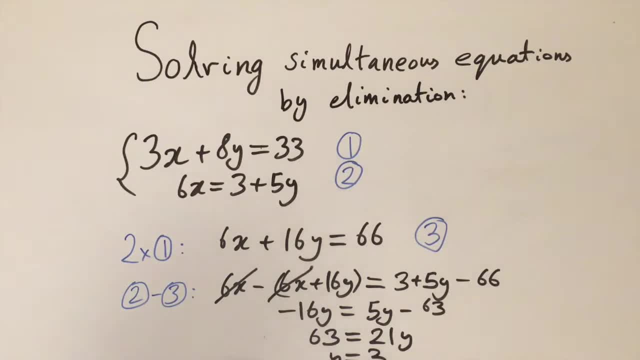 solution. So now our second step is to substitute this value of y into one of the original equations and use this to find the variable x. And that's the second half of the solution. So let's substitute, So we get y into the first equation. This is the simplest, And let's go up here And 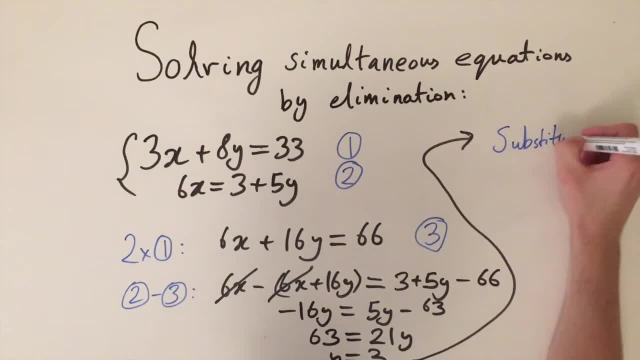 let's write substitute in 1.. OK, So we have 3x- That's what we were trying to work out- And 8y. So plus 8.. And y is equal to 3.. So 8 times 3. And this is equal to 33.. So all. 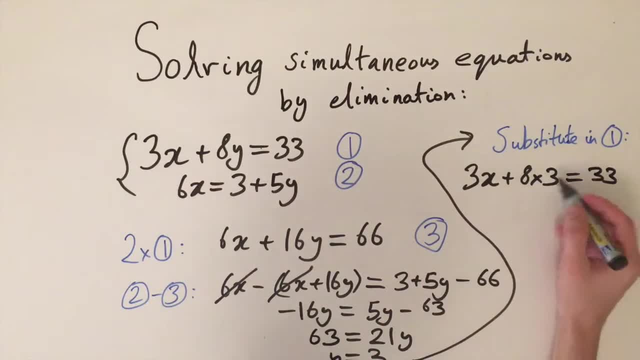 we've done is substitute the variable. So we've just substituted the value of y into the first equation And now we can solve this. We have: 3x is equal to 33 minus 8 times 3.. 8 times 3 is 24.. So I've just moved that onto.